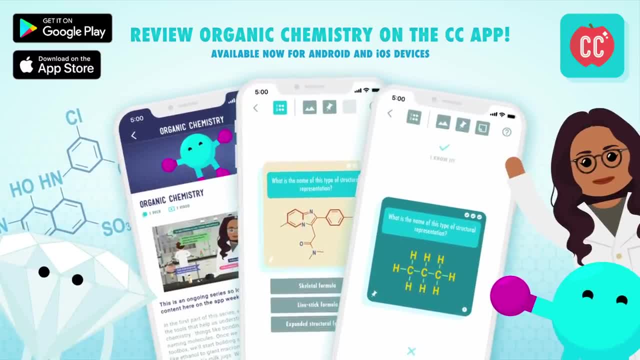 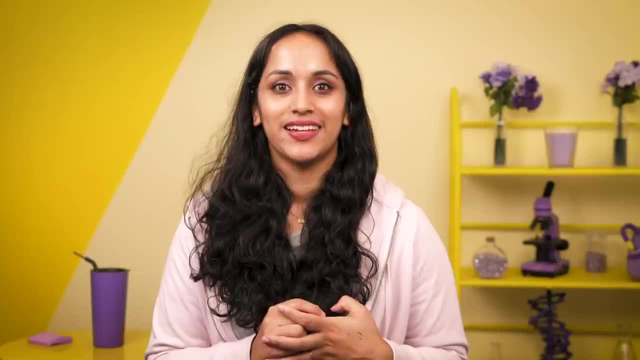 You can review content from Crash Course Organic Chemistry with the Crash Course app, available now for Android and iOS devices. Hi, I'm Deboki Chakravarti and welcome to Crash Course Organic Chemistry. Chemists used to have a real problem when it came to identifying the crystals. 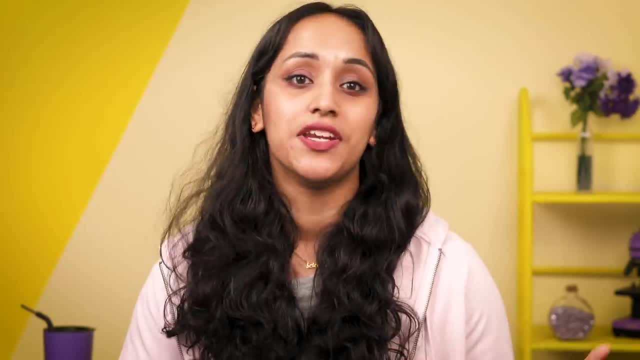 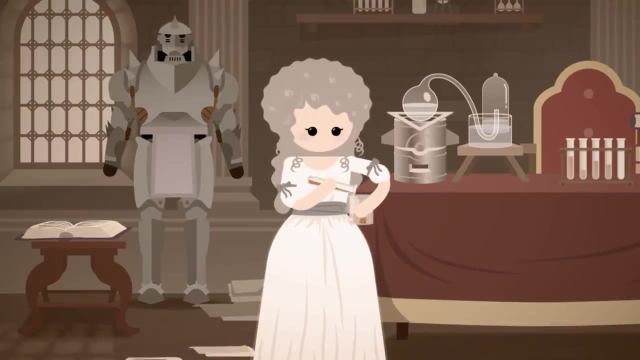 liquid or general gloop they found themselves with at the end of a chemical reaction. Of course they knew what they were trying to make, but had they actually made it? They could check boiling points, melting points, smell, color or even taste in the bad old days. 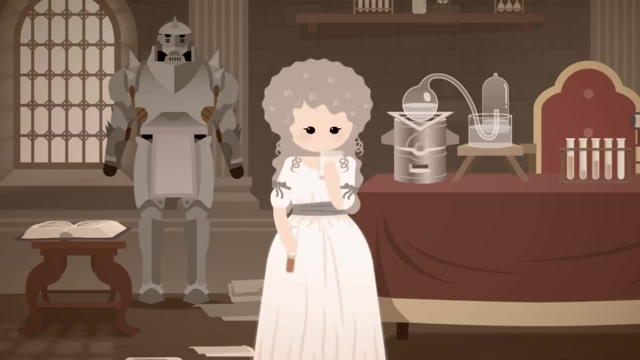 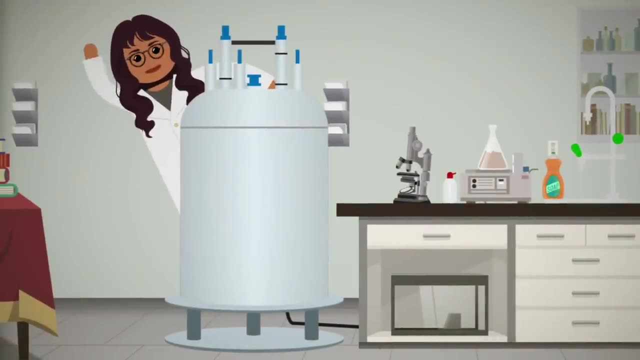 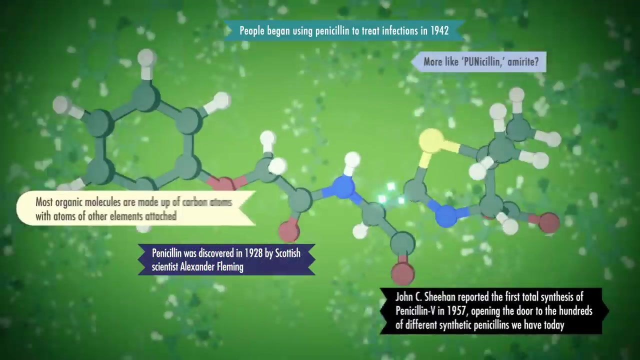 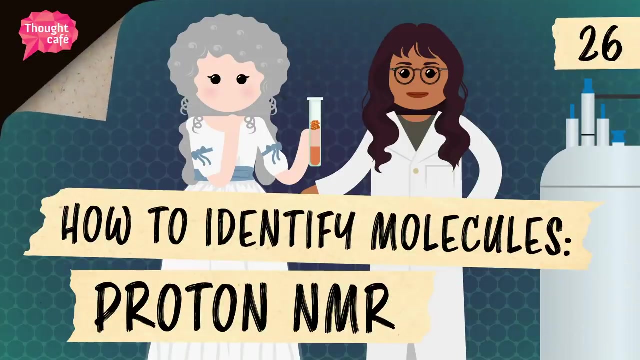 which is definitely not recommended now. But all of that took weeks of diligent effort and was still somewhat inconclusive. Fortunately, we've moved on to a much more high-tech analytical technique: Nuclear magnetic resonance or NMR. First off, let's straighten one thing out. 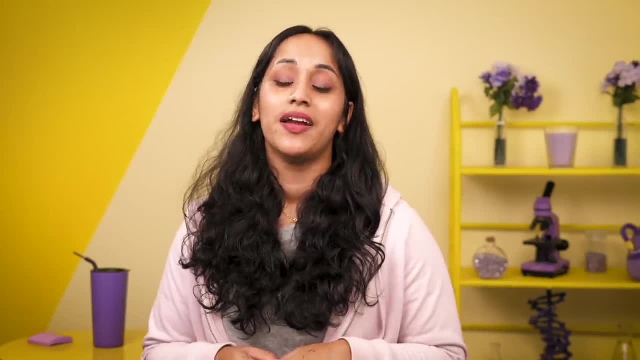 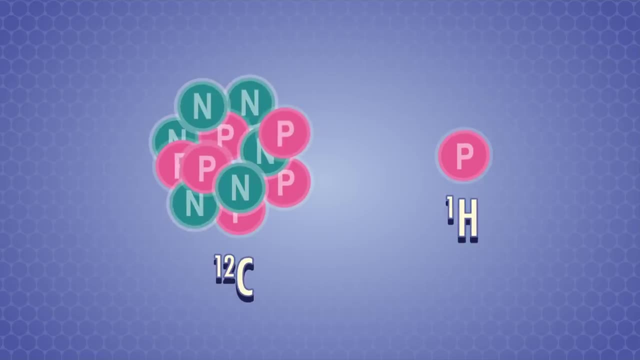 The nuclear part of NMR's name doesn't refer to nuclear power. It refers to the nuclei of atoms. All atomic nuclei are made up of protons and neutrons, except for hydrogens, which doesn't have any neutrons. Adding up the protons and neutrons gives us the atom's mass number. 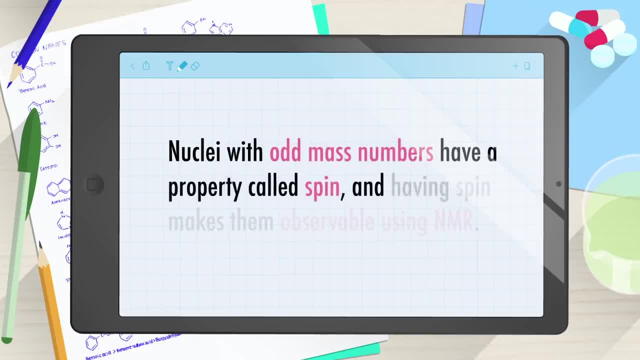 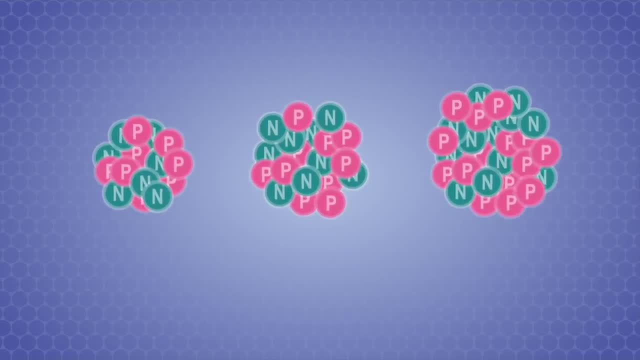 Nuclei with odd mass numbers have a property called spin, and having spin makes them observable using NMR. Obviously, there are quite a lot of elements with odd mass numbers, but we're only interested in a handful of them for NMR. 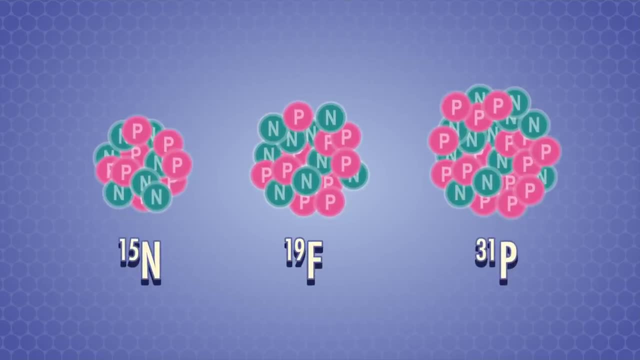 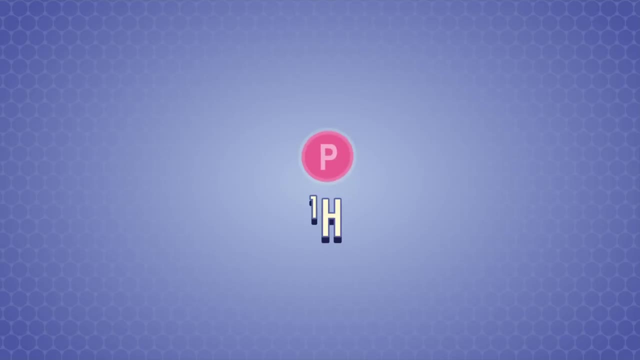 Nitrogen-15,, fluorine-19, phosphorus-31 all show up occasionally, but the real stars are carbon-13 and hydrogen. We'll focus on hydrogen today and do proton NMR. Spin is not the nuclei literally spinning, It's one of those weird quantum mechanical things. 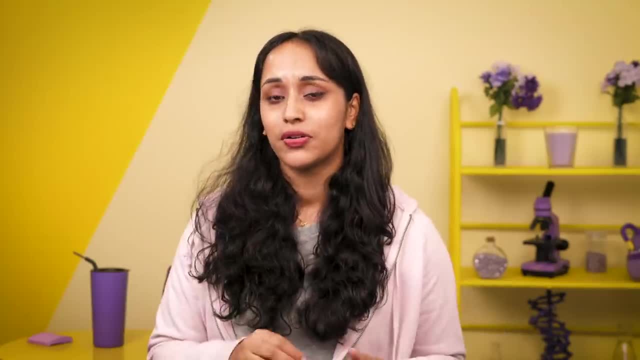 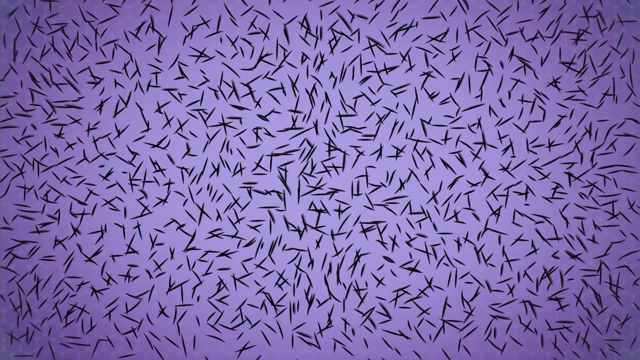 To avoid getting too into the physics, we'll just say that when charged particles like protons in a nucleus move, a magnetic field with a magnetic moment is created. If you've played with iron filings before you know they move if you put a magnet near them. 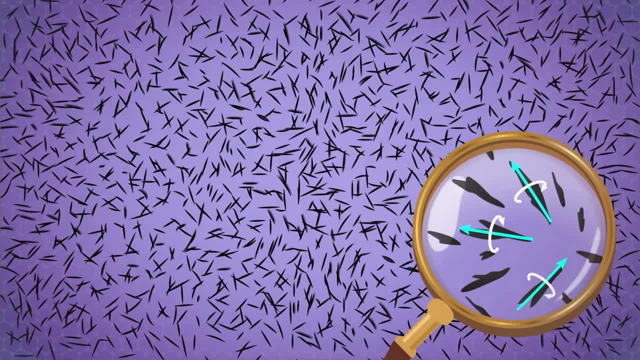 Either way they move when you put a magnet near them, Either way they move when you put a magnet near them, Either way they move when you put a magnet near them. Each iron filing has a magnetic moment and under normal circumstances their directions are random. 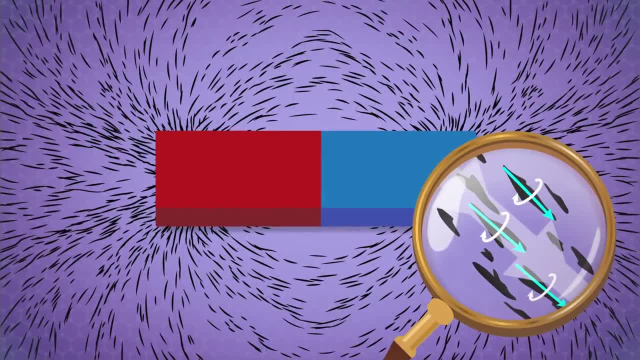 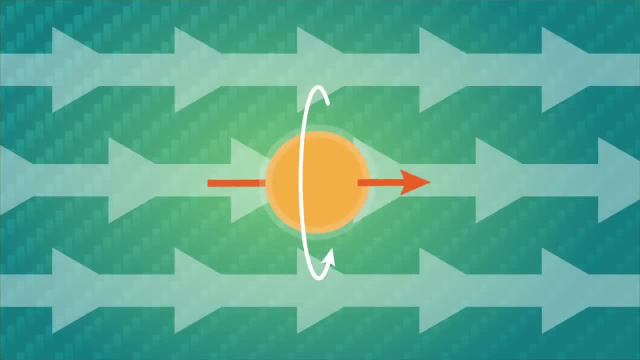 However, in the presence of a magnet which has a magnetic field, they all line up. Similarly, if you stick a nucleus with a magnetic moment in an external magnetic field, it either lines up with that field or exactly against it. It takes less energy to align with the magnetic field and more energy to go against it. 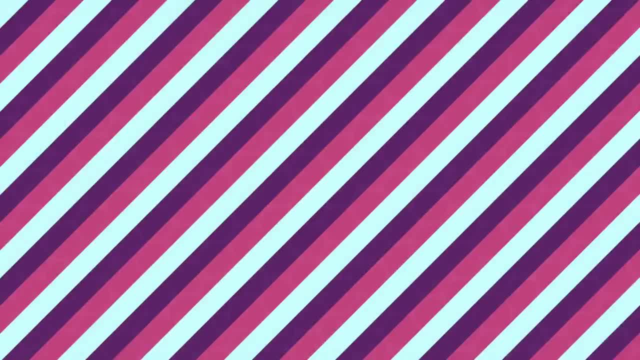 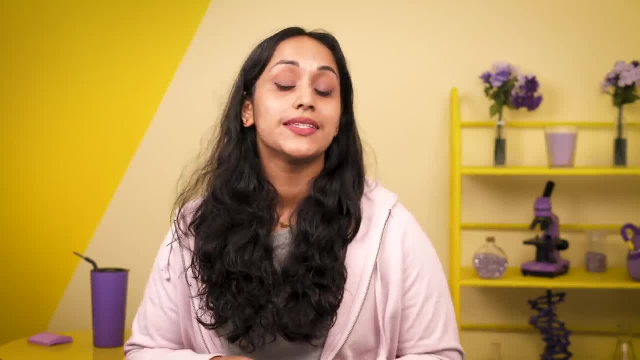 so there's a clear energy difference between the two different spin states. Now we've got the nuclear and magnetic parts of NMR covered, but what about the resonance? It turns out that particular frequencies of radio waves will cause the nuclei to flip from one spin state to the other. 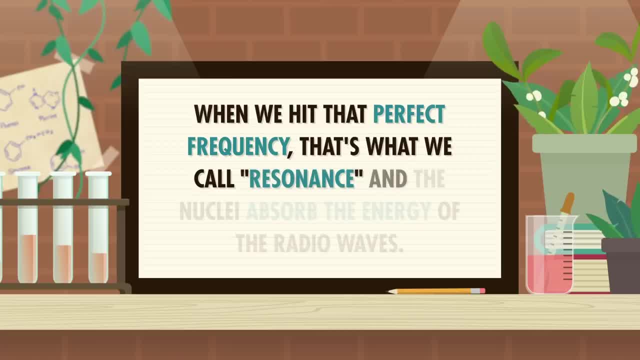 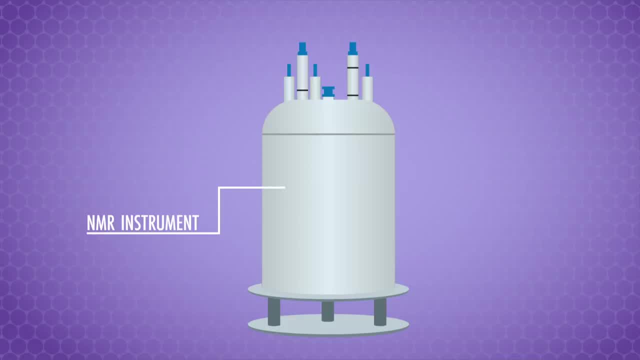 When we hit that perfect frequency- that's what we call resonance- and the nuclei absorb the energy of the radio waves. This is where a detector measures the frequency and intensity of the radio wave that got absorbed and plots it on a spectrum. In this episode, we're going to concentrate on proton NMR. 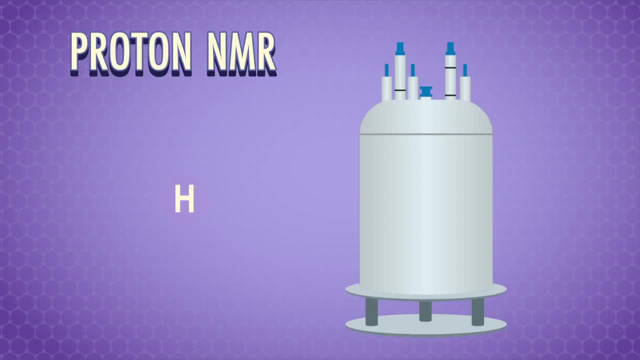 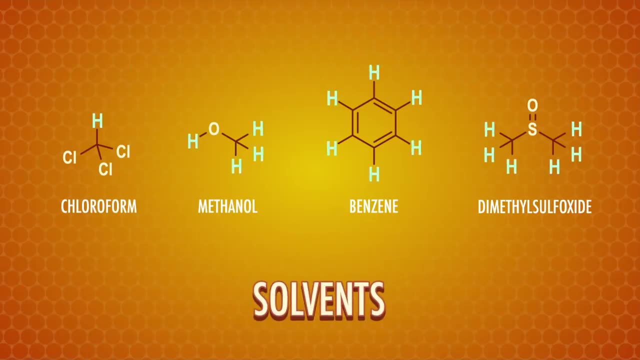 which tells us about the hydrogen nuclei and therefore hydrogen atoms in molecules In general. we'll get a huge magnet and dissolve our chemical sample in a special deuterated solvent where the hydrogen atoms are replaced by deuterium. If we used a regular old solvent with protons, 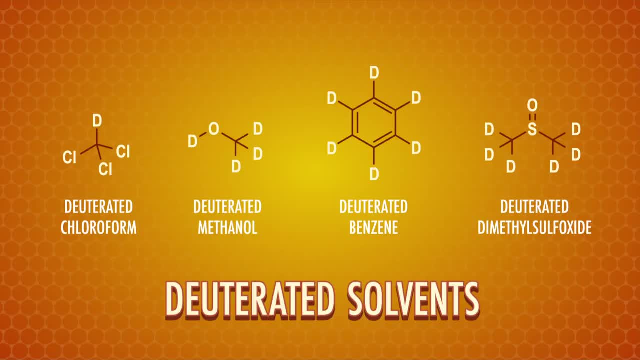 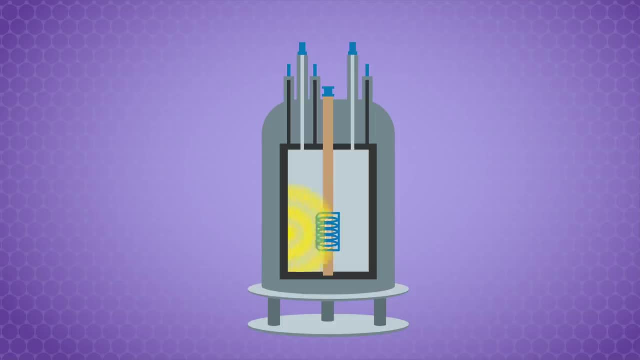 the signals from our organic chemical would be overwhelmed by the hydrogens on all the solvent molecules. Then we put our tiny solution of chemical sample in the middle of the magnet, blast a pulse of radio waves and measure the energy released by the nuclei as the different hydrogen atoms in the chemical go from resonance back to their ground state. 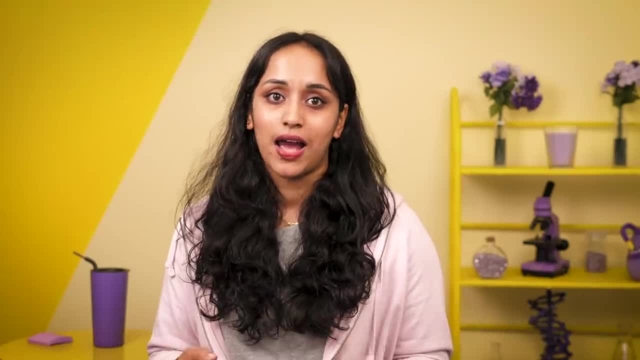 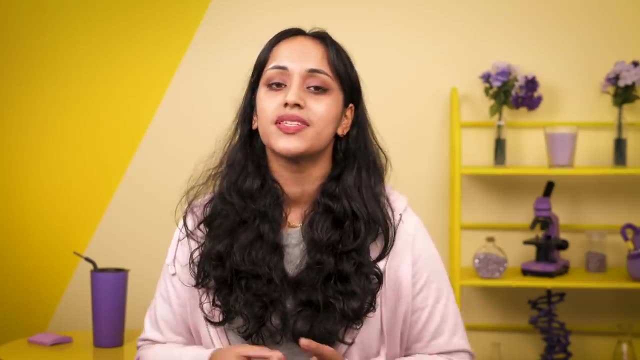 Like IR spectroscopy that we talked about in episode 5, we get a spectrum from the sample. Once we look at some proton NMR spectra, we'll get the hang of these patterns. Let's start with a simple example. This is the spectrum for chloromethylmethylether, or mom chloride to its friends. 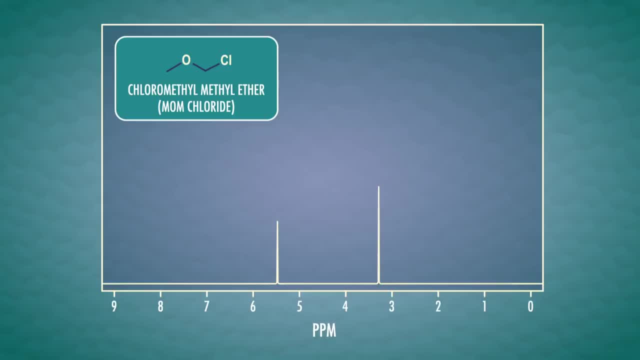 The x-axis is measured in ppm, which stands for parts per million. It has to do with the ratio between the radio frequency source and the energy required to cause the nuclei to flip spin. The process of adding deuterium to solvents isn't perfect. 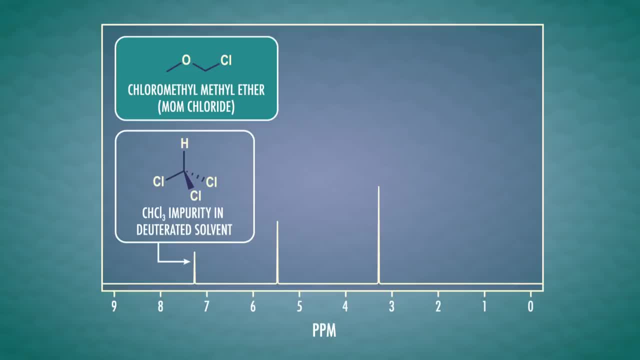 so a few hydrogens from the NMR spectrum will be used to measure the radio frequency. We can also use a standard chemical called tetramethylsilane or TMS in the sample, which produces a very strong signal. TMS shows up on the far right of the spectrum and usually doesn't overlap. 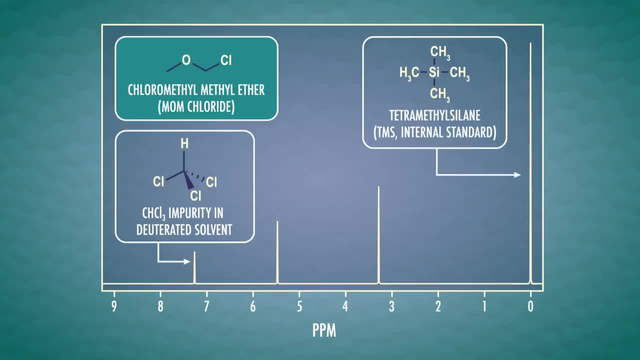 with the peaks from the hydrogens on our organic chemical. Basically, the standard provides a comparison point for the other peaks. It's a bit like measuring times against GMT. If you live in New York, your time zone is GMT-5,, while your time zone is GMT-1.. So if you live in New York, your time zone is GMT-5,, while someone in Paris is on GMT-1, and someone in Canberra, Australia, is on GMT-11.. So ignoring the peak at zero from our TMS standard. 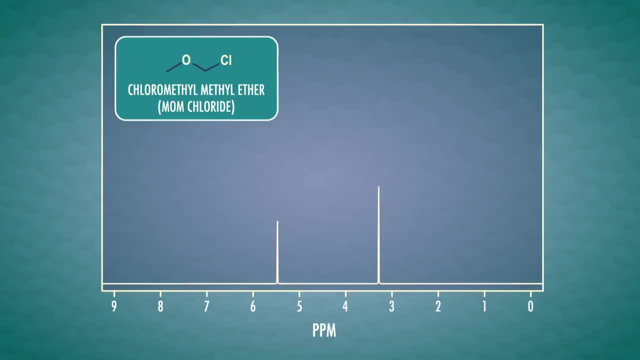 there are only two peaks we need to analyze in the spectrum. Using a computer, we can label each of these peaks with the integral, the area underneath them, which corresponds to the ratio of the number of protons in that part of the molecule. 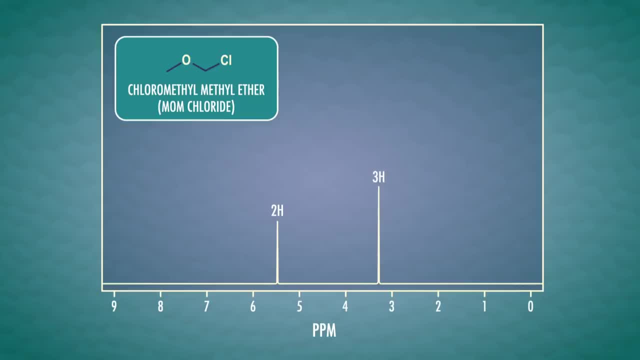 One of our peaks here has an integral value of 3,, which means three protons. So that means there's probably a methyl group- CH3, in our sample. The other peak has an integral of 2,, which suggests our chemical also contains a CH2 group. 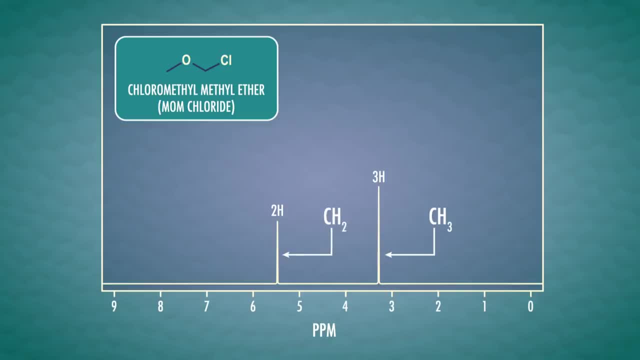 So if we were a chemist in a lab who didn't know, but just suspected that we had mom chloride, we could check whether the structure of our suspected molecule fits with our spectrum. And yep, there sure is a CH3 and a CH2 group in mom chloride. 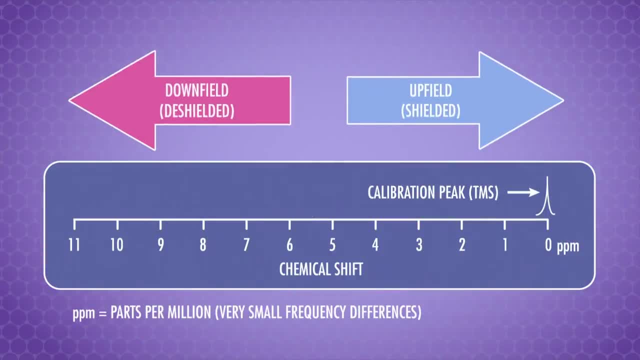 One of the peaks is upfield or further to the right, and the other is more downfield or further to the left. That's because the protons making up these peaks are surrounded by different amounts of electrons because of different neighboring atoms. 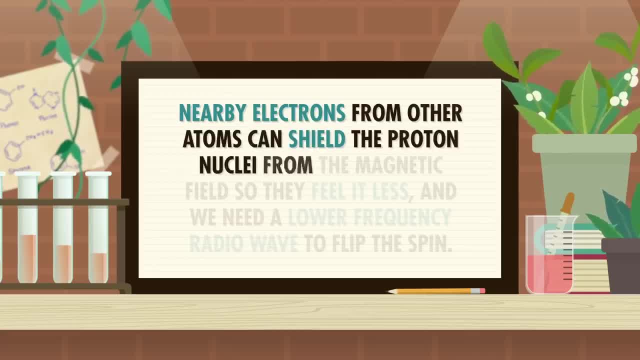 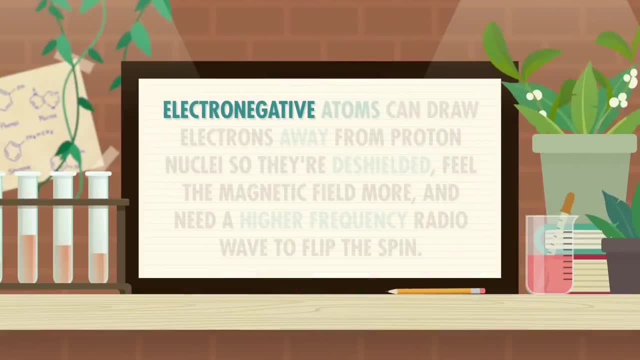 Nearby electrons from other atoms can shield the proton nuclei from the magnetic field, so they feel it less and we need a lower frequency radio wave to flip the spin. On the other hand, electronegative atoms can draw electrons away from proton nuclei. 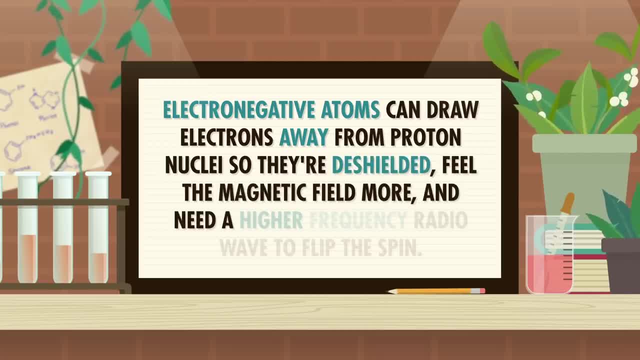 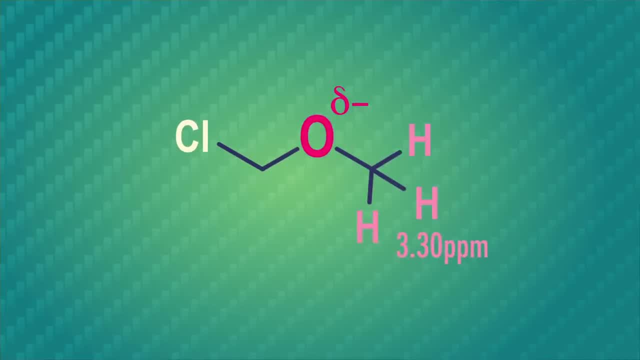 so they're deshielded, feel the magnetic field more and need a higher frequency radio wave to flip the spin. Taking a look at mom chloride, we can see the CH3 group is attached to an electronegative element, oxygen. 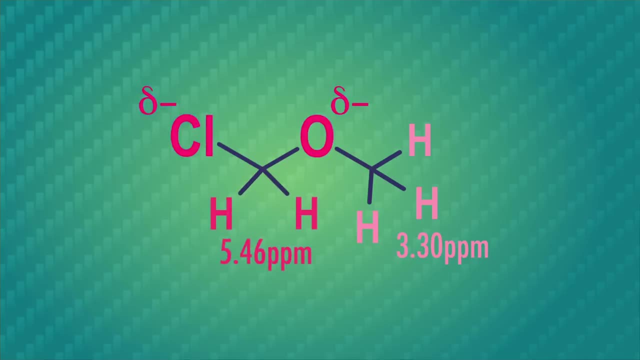 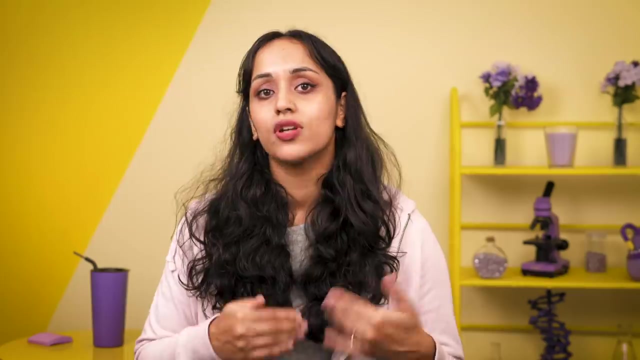 But the CH2 group is sandwiched between two electronegatives, an oxygen and a chlorine. So the electrons near the CH2 groups are more drawn away, the proton nuclei are more deshielded and the peak is downfield of the CH3 group. 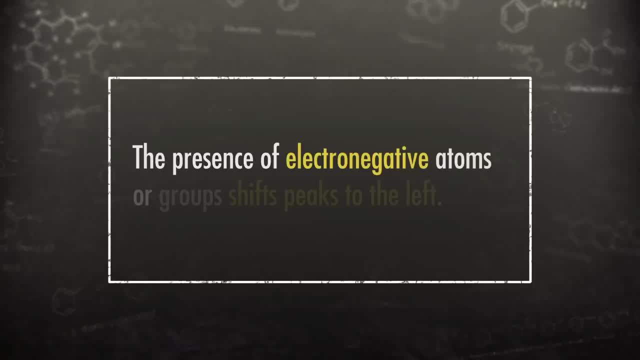 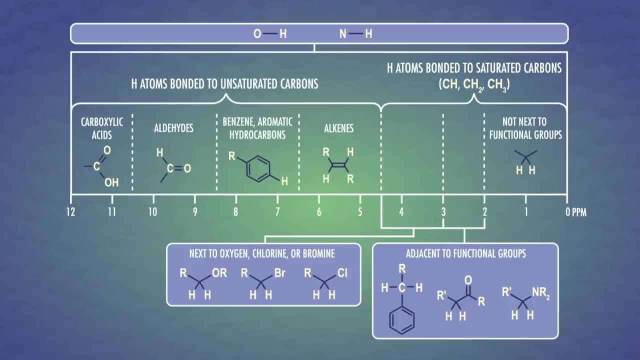 To keep it really simple, just remember that the presence of electronegative atoms or groups shifts peaks to the left In proton NMR. the peaks on the spectrum actually have pretty consistent shifts based on the electronegativity and hybridization of the atoms near the protons. 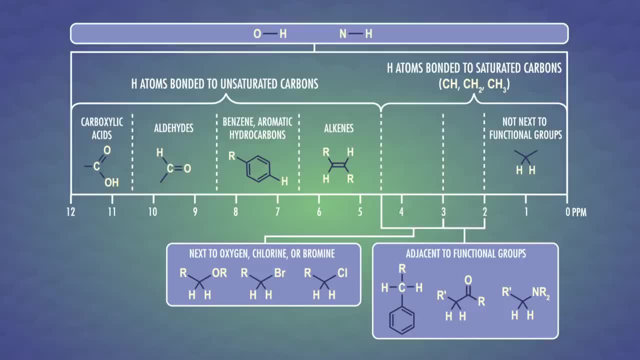 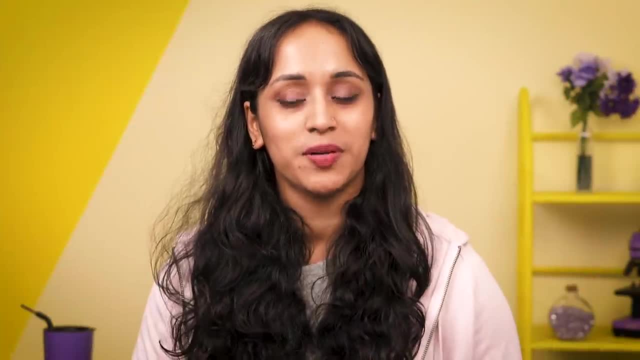 Tables like this can't cover every possibility, though, which is why we need to understand how to think about electronegativity and chemical shift. Okay, now that we've talked through the mom chloride spectrum, let's try another example. This is the proton NMR spectrum of ethanol. 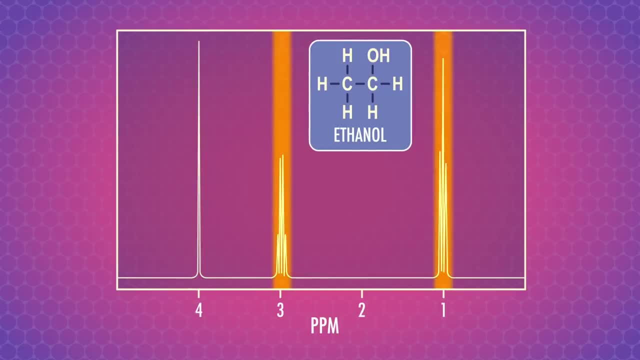 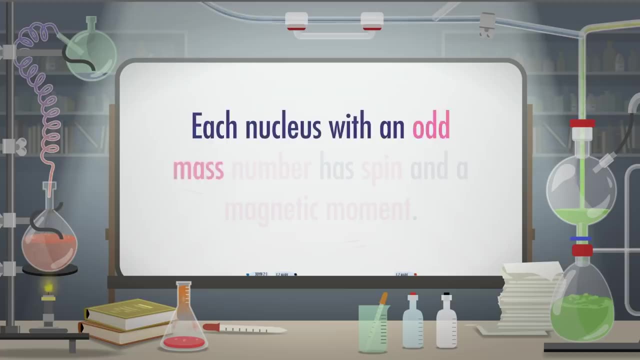 There are three peaks in this one, But two of them are more like… groups of lines. There are lots of protons in organic molecules, and remember that each nucleus with an odd mass number has spin and a magnetic moment. So protons on one carbon can influence protons on an adjacent one. 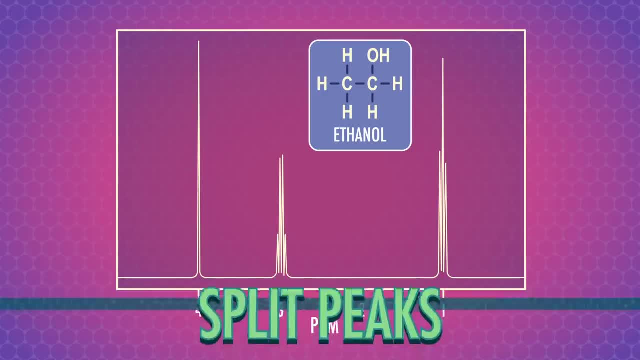 and protons on another carbon can influence protons on an adjacent carbon in a process called coupling. This leads to the split peaks, or groups of lines that we're seeing here. In fact, this has been observed so regularly that we can predict how many times a peak will be split. 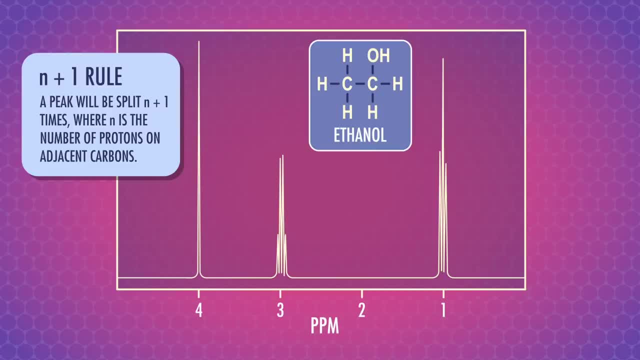 Thanks to the aptly named N plus 1 rule, we know that a peak will be split N plus 1 times, where N is the number of protons on adjacent carbons. The best way to understand splitting is by looking at examples. 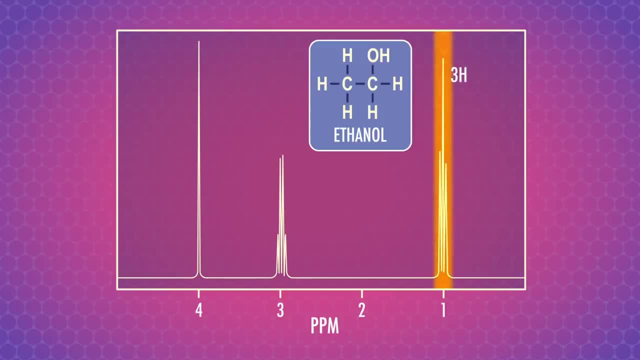 So let's start with our most shielded peak. It's at about 1 ppm with an integral of 3, so it's about 1 ppm. So we know it's the CH3 group. We're still practicing. so let's look at the structure of ethanol. 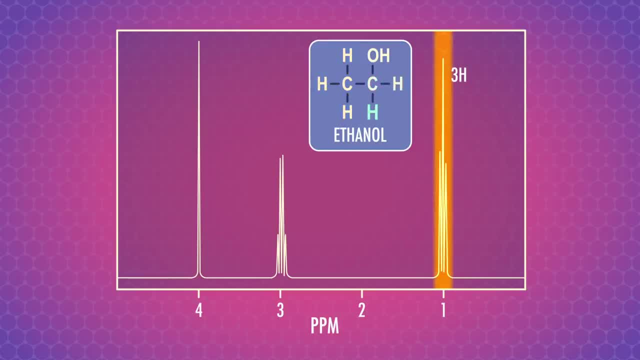 The CH3 group is bonded to a CH2 group. There are two protons on the neighboring carbon that are coupled. This means N is 2.. Using the N plus 1 rule we can do: 2 plus 1 equals 3, so the CH3 peak should be split into 3.. 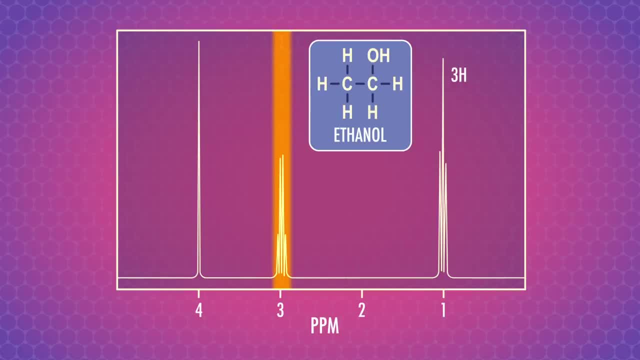 Now going one peak downfield, at about 3 ppm we see the CH2 group in our spectrum. It's downfield of the CH3 because the CH2 group is bonded to an electronegative atom In the structure of ethanol. we know that the CH2 group is bonded to the CH3 group. 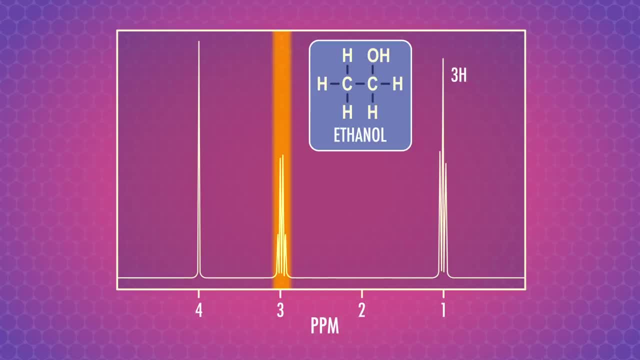 so there are three protons on the neighboring carbon that are coupled, and N is 3.. Using the N plus 1 rule, 3 plus 1 equals 4, so the CH2 peak is split into 4.. Plus it has an integral of 2, telling us there are two protons. These split peak patterns or multiplicities have special names too. The CH3 peak split into 3 is a triplet and the CH2 peak split into 4 is a quartet. The third peak split into 3 is a triplet and the CH2 peak split into 4 is a quartet. 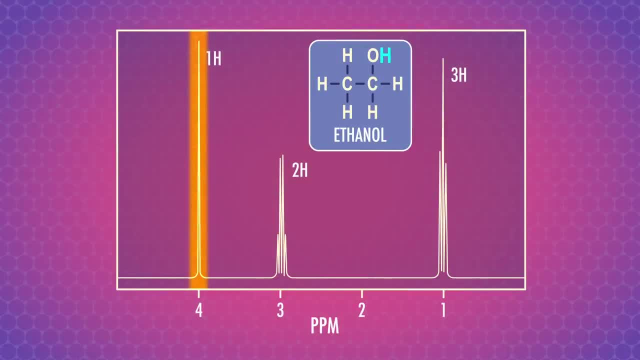 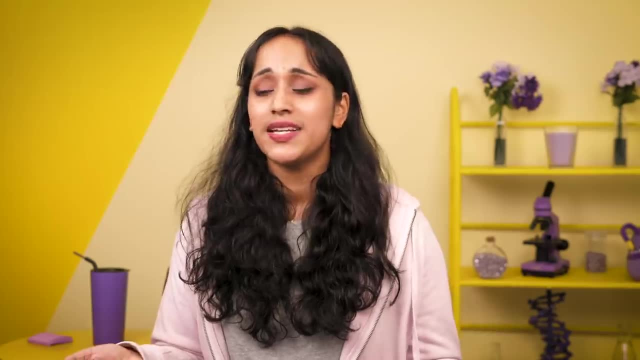 The third peak, at about 4 ppm, is the proton on the OH group of our ethanol molecule. OH protons are tricky because they can swap with other protons in the sample solution and can turn up as unsplit peaks pretty much anywhere in the spectrum. In fact, sometimes they don't show up at all. It's also important to mention that the protons on oxygen and nitrogen don't split the protons on adjacent carbons, so these protons don't count when figuring out N plus 1.. 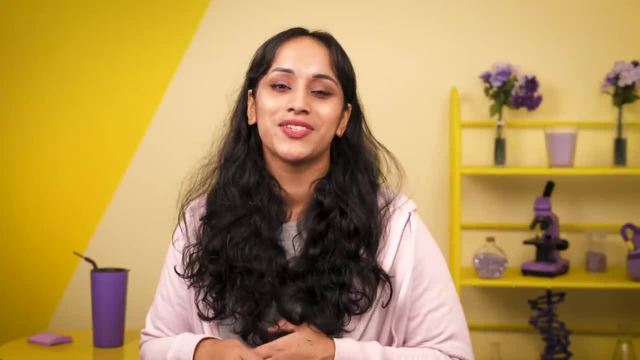 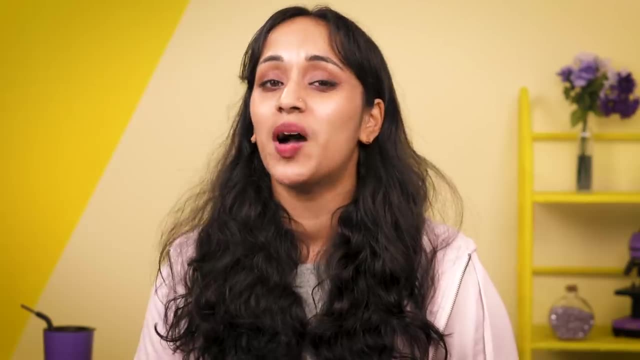 After you look at more peaks and more spectra. solving these logic puzzles can be fun. And because the whole point of proton NMR is to figure out the structure of molecules. this next spectrum doesn't come with a named structure like mom chloride or ethanol. 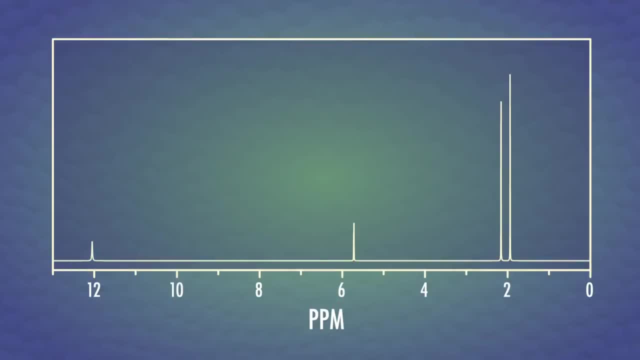 Fortunately, we have a high-resolution mass spectrum that gives us our chemical formula C5H8O2.. So let's start with the most shielded part of the spectrum. We have two single peaks that have integrals of three protons each. 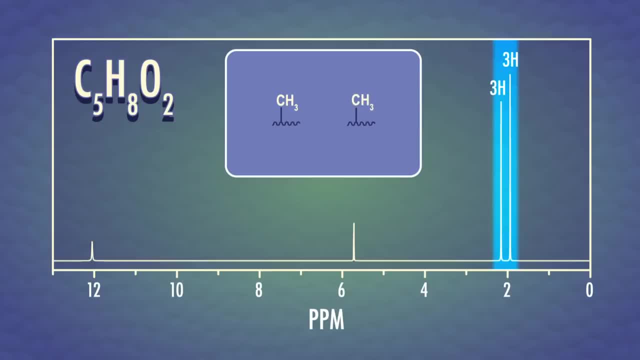 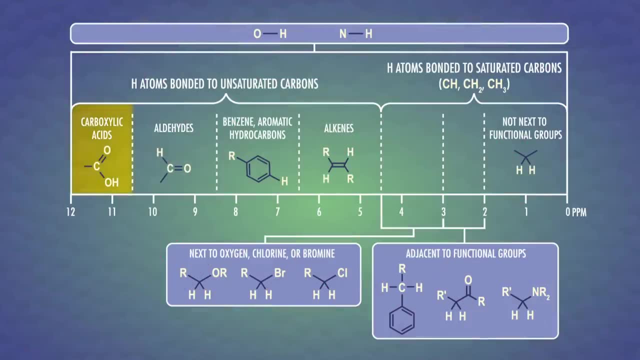 so it looks like we have two CH3 groups on our mystery molecule. Next, we can see that the most deshielded single peak has an integral of one proton. Referring back to our handy chart, we can see this is where the proton on a carboxylic acid shows up. 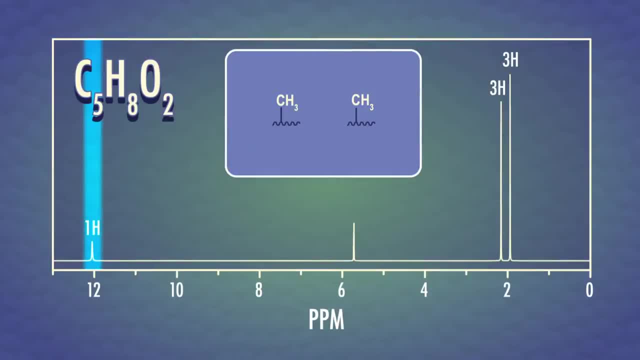 And what do you know? we have two oxygen atoms in our formula, which fits perfectly with that thought. Let's add this fragment to the pieces of our molecule puzzle. One more peak to go, and this single peak corresponding to one proton. 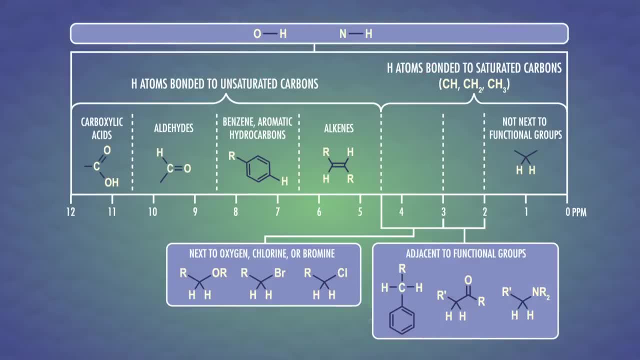 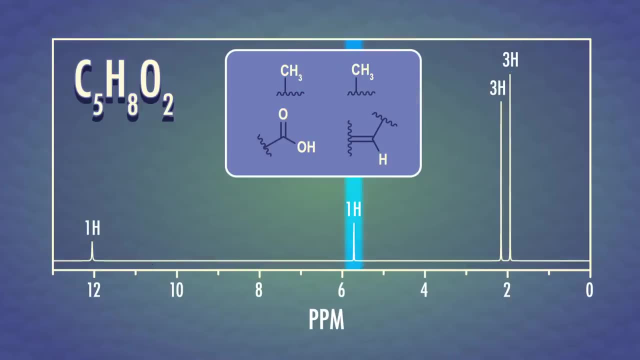 is a bit deshielded too. In fact, looking at our chart again, it's showing up in the range of alkene hydrogen atoms. The trickiest part about putting these four pieces together is figuring out where to place the two methyl groups and the carboxylic acid on our alkene. 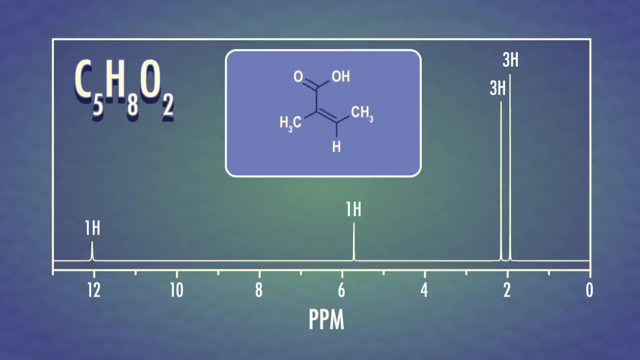 To start, let's put the two CH3 groups on different sides of the alkene. Wait a second, though. With this structure, the methyl group is next to a carbon atom with a hydrogen. This would split a single peak into a doublet. 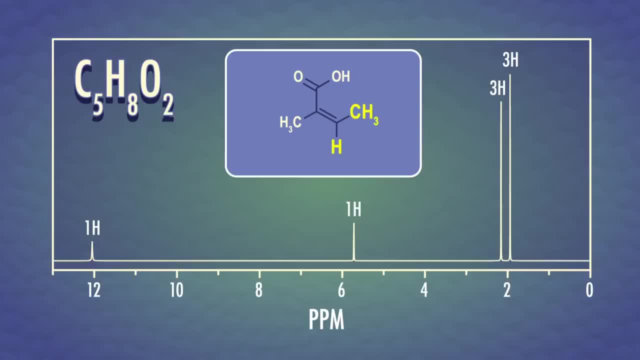 and we'd expect the hydrogen atom to be split by the three hydrogens, on the methyl too. Since we don't see splitting in the spectrum, let's rearrange our structure so the hydrogen atom and both methyl groups won't be split by any adjacent protons. 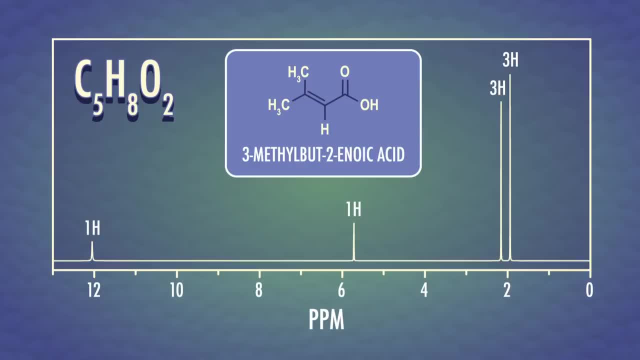 Even though the two methyl groups are attached to the same carbon, double bonds are rigid, So one of these groups is stuck on the same side as the carboxylic acid and one is on the same side as the hydrogen. These methyl hydrogens are in different chemical environments. 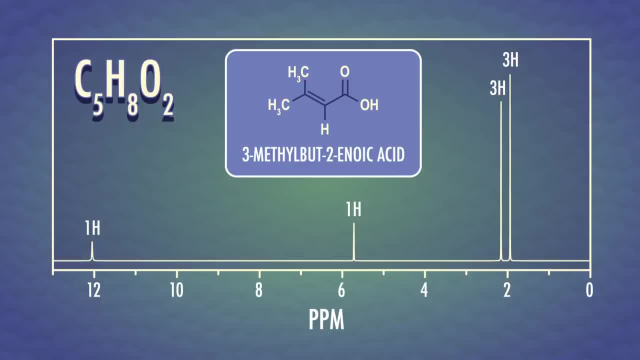 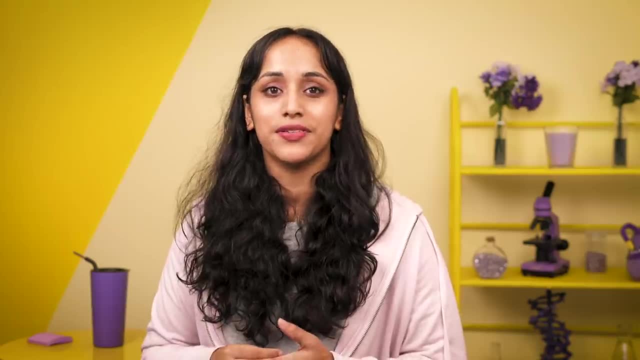 and they're not chemically equivalent, so that's why they show up as two different peaks. We'll talk more about chemical equivalents in a later episode when we look at the proton NMR spectra of aromatic compounds, But in this episode we've learned nuclear magnetic resonance helps us.